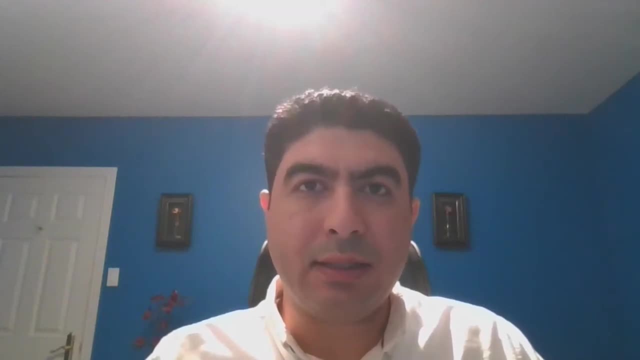 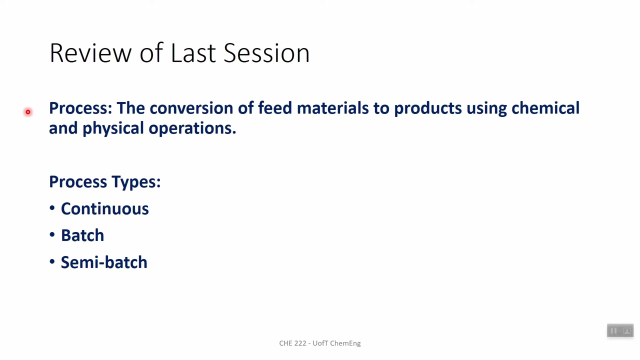 Hello everybody, This is our first asynchronous lecture and our second lecture in total. I'll give you a review of the previous session and then we start a new topic. In the previous session I defined a process and identified three process types. Then I gave you a general perspective of the 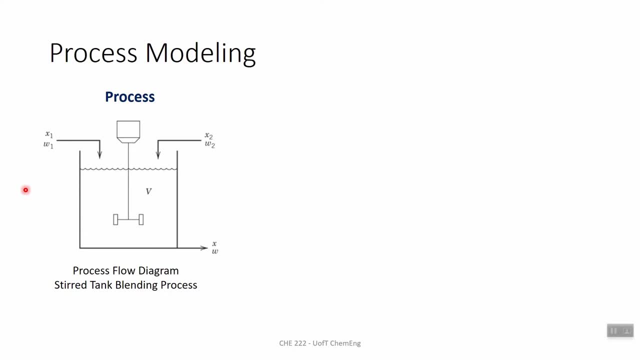 objective of this course, which are three different steps basically. First is process modeling, and process modeling is basically representation of a process with mathematical equations, and they can be done for two different states of the process: a steady state and transient state. Once we have these, 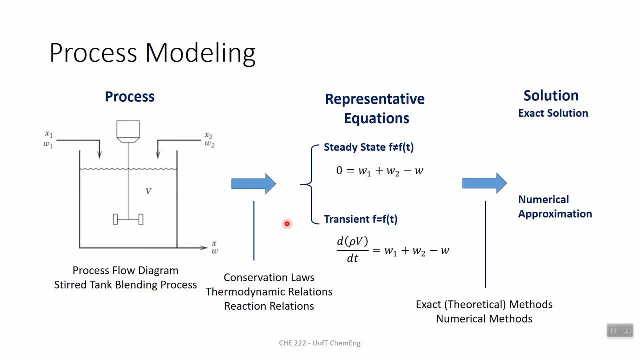 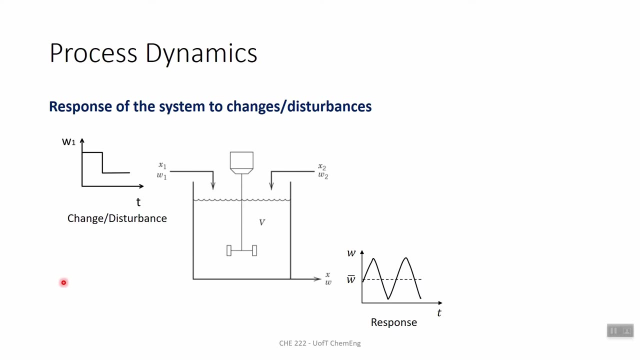 mathematical equations. next is to solve them using exact methods or numerical methods. Now let's say we have an equation for the transient state of a system. Then we can get into process dynamics, which is the response of the system to changes or disturbances, normally with respect to 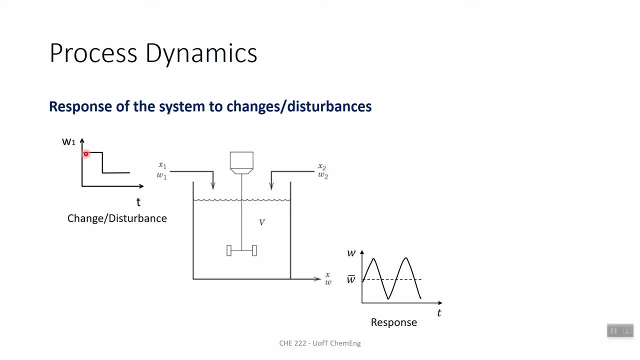 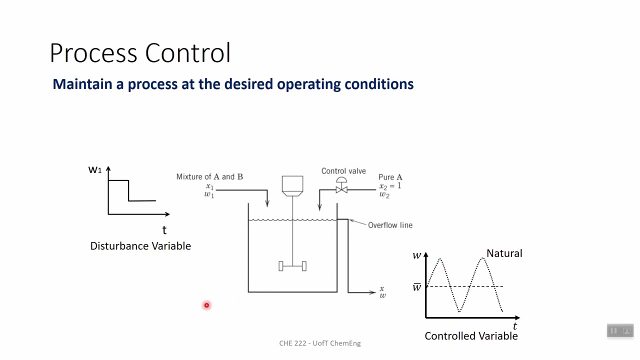 the time. For example, let's say we have a variable or an input variable that varies with time, like this step function, Then how does the output of the system or the response of the system vary with time? and finding this is part of process modeling. Now that we find this, our next goal is to basically control the process. 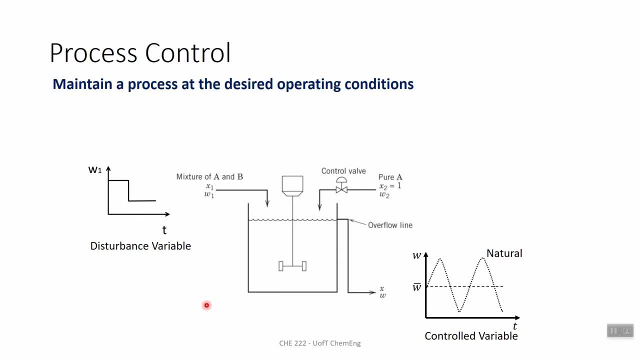 so that we can maintain a process at the desired operating conditions. Let's say, our desired operating or output condition is this uniform level. But we know a small change in the input variable may result in a large fluctuation. So to solve this we have to. 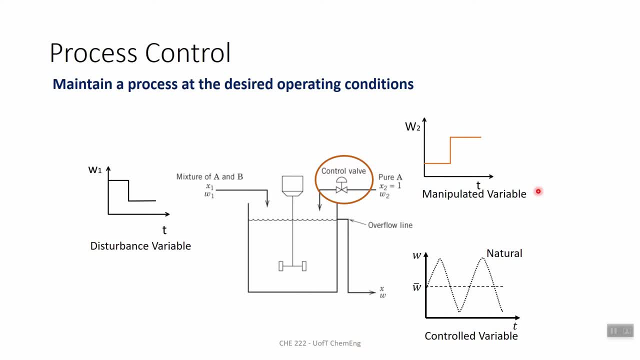 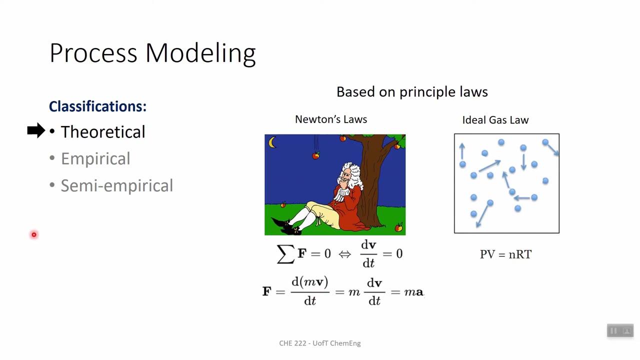 start with a way to control the system, so that at least our fluctuation with respect to the time are within an acceptable range. Now let's start the topic of this session, which is process modeling. There are three different types for process modeling: Theoretical, empirical and semi-empirical. 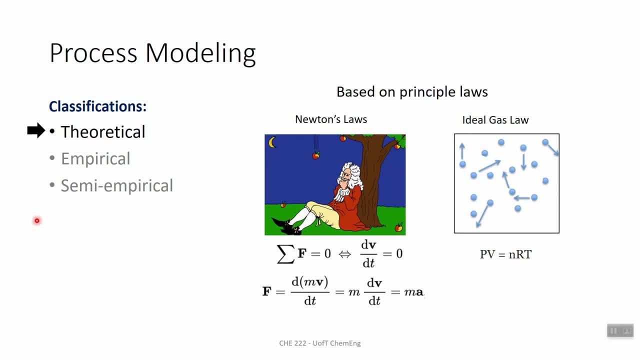 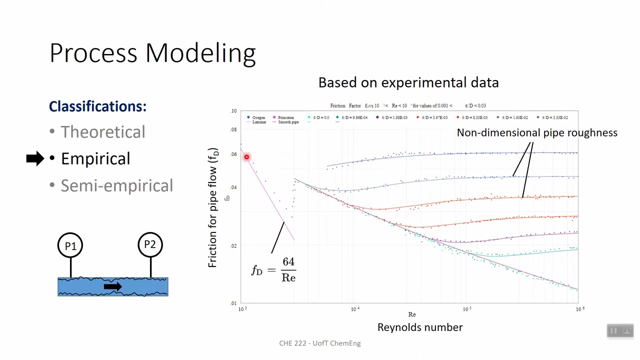 For this course. we will mostly use theoretical modeling, which is based on principle laws, Something like Newton's law or ideal gas law- which relate any physical or chemical phenomena to some sort of mathematical equations. There is also empirical modeling, which is based on experimental data, So you have to obtain a lot of data points and then 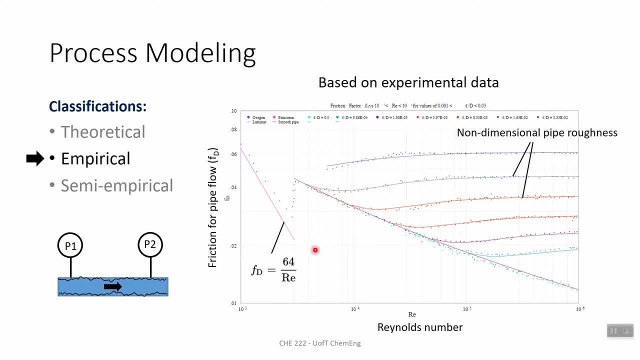 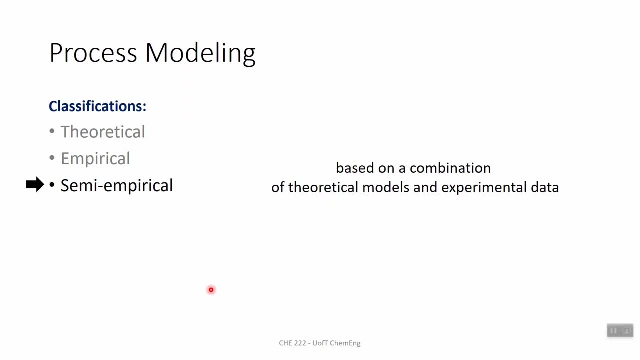 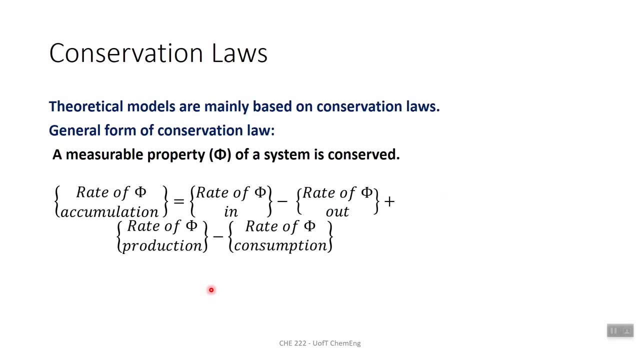 start carefitting these data points to come up with a correlation for the desired parameter. And finally, there is semi-empirical method, which is based on a combination of theoretical models and experimental data. But, as I said, in this course we will mostly use theoretical modeling. 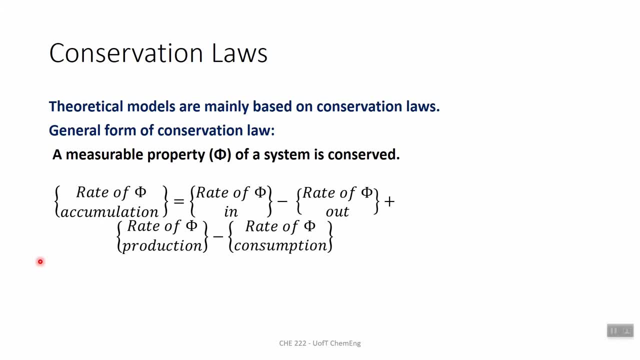 which is based on conservation laws. We can write a general form of conservation law for an arbitrary property of the system. Let's call it phi. So if my system consists of a control volume, the rate of phi into the system minus the rate of phi. 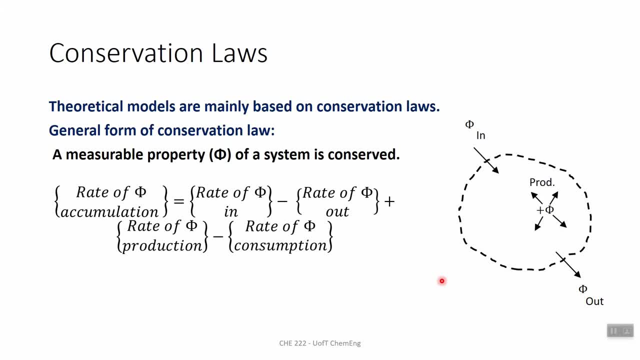 out of the system, plus the rate of production or generation of phi within the system, minus the rate of consumption of phi within the system, defines the rate of accumulation of phi, which is basically d, phi over dt or time. So this is the general form of conservation law and we will apply this to different properties. 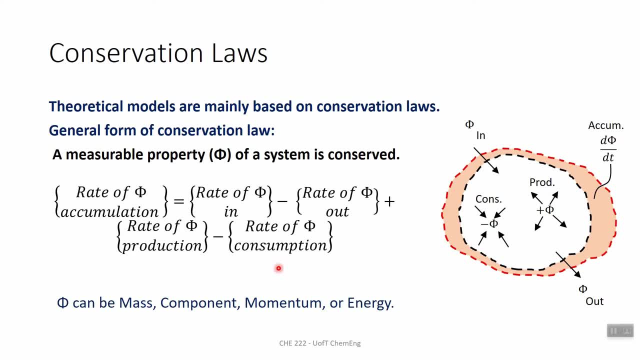 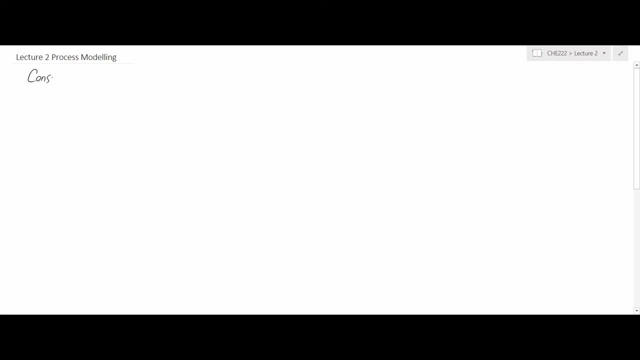 of systems, including mass, component, momentum or energy. next, Okay, let's now drive the conservation of mass. For that we have to set phi equal to 0. equals to mass, and we had for the general form of conservation law. we had the rate of accumulation of a certain property, which is, in this case, mass, is equal to rate of mass into our system. 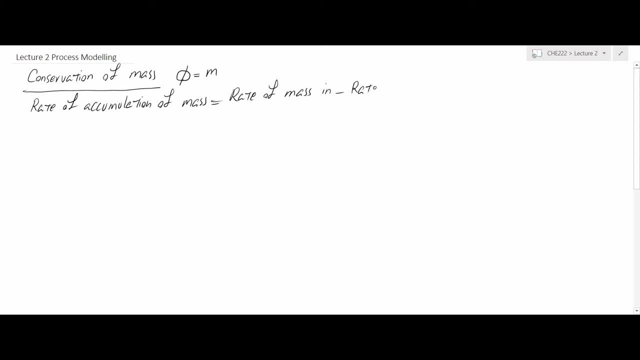 minus rate of mass out of our system, plus rate of mass production, minus rate of mass consumption, and we know that we cannot produce or consume mass. so these two last terms are zero and we're left with rate of accumulation of mass. so just to make it more, 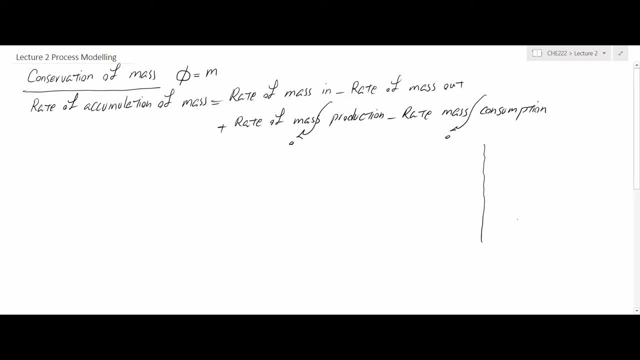 understandable. I give you this example of blending tank with an agitator in the middle and we have two input streams into the tank: one at the flow rate of Constitution and other instruments. we are Sunny Bay. we are gonna also be considering all soon is Helloản. 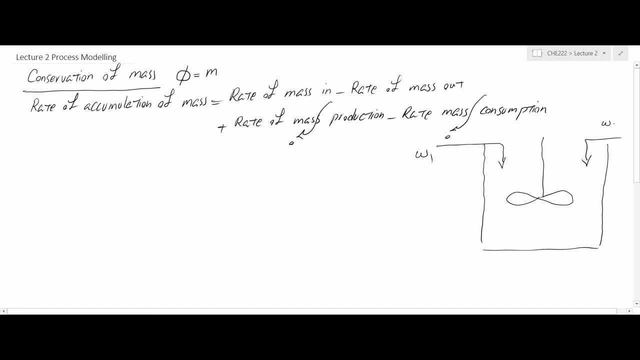 W1 and the other one and the flow rate of W2, and these are mass flow rates. there's a level of liquid within the tank and I intentionally put the discharge of the tank at an elevated location and I assume that it is large enough that can handle the two input streams. so it means that for now, the 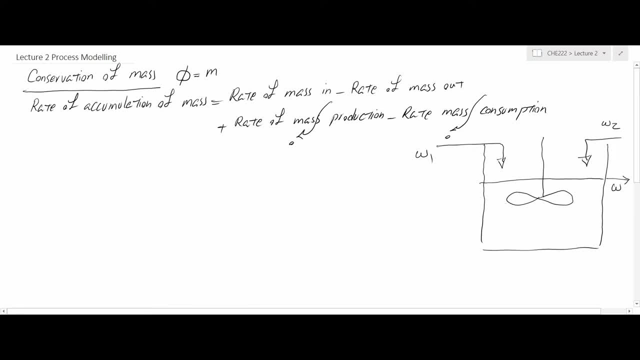 amount of liquid within the tank is constant. so if I rate, if I convert this into mathematical form, rate of accumulation of mass is a derivative of mass mass with respect to time, B MDT, rate of mass into the tank- and I assume this tank is my basically control value is W1 plus W2. a rate of mass into 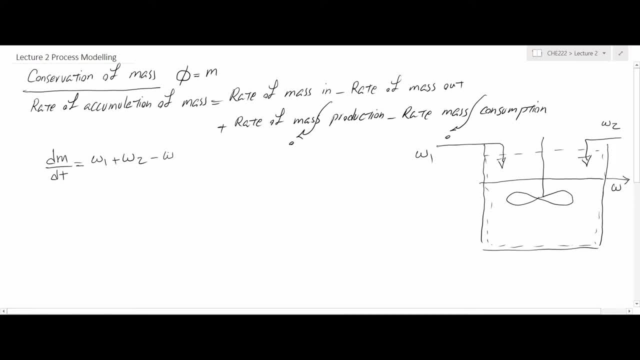 the tank minus W, which is rate of mass out of tank. so as I said in the first, we assume in the case that discharge is an elevated location, it's an overflow and it's large enough to handle the two input streams. so in that case the amount 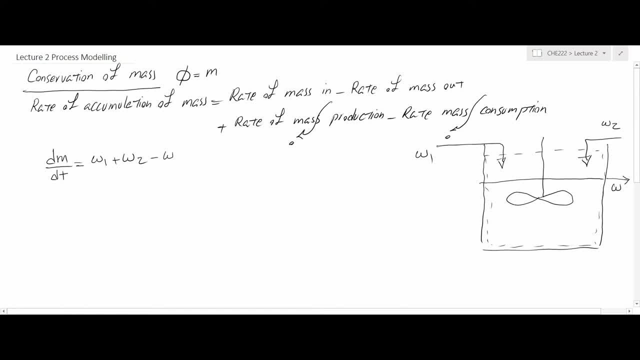 of liquid within the tank stays the same, because whatever comes in goes out and we can assume that basically we don't have any accumulation of mass within the tank. so the equation becomes zero. equals to W1 plus W2 minus W, which is basically our mass conservation in a. 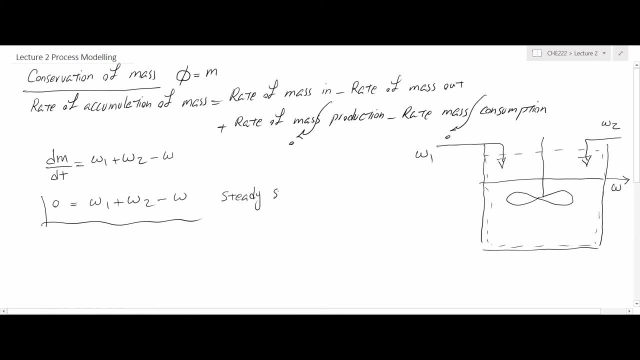 steady state. but if I go ahead and delete this and put it down below and I write the Equal性 and I add a valve in here so I can throttle the flow, so there is a valve and with this valve I can play with the basically opening of the orifice and I 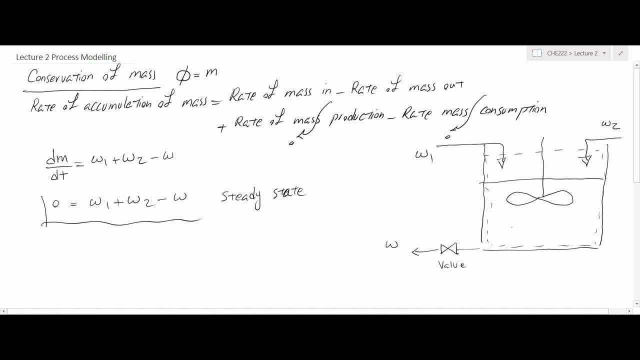 can manipulate the outlet of the system and with that I can either accumulate some mass within this tank or let the amount of liquid within the tank to reduce. so in that case we have the derivative of mass with respect to the time, and if I replace it with the density of liquid times the volume of liquid within the time, I will. 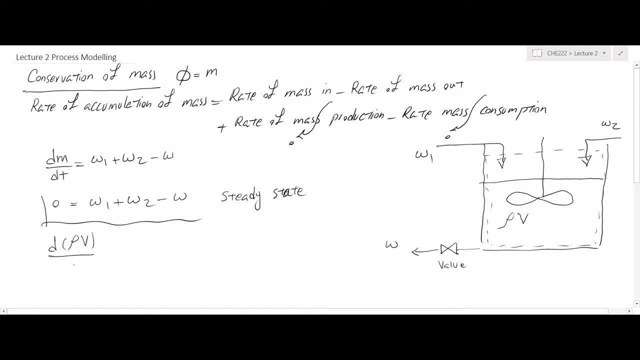 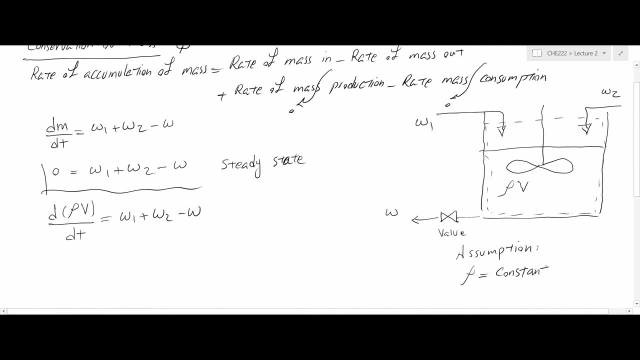 have d rho times V, divided by t, dt or derivative of rho V, and with respect to time, is W one plus W, 2 minus W. and now I can make my first assumption here, which is basically rho is constant and this is not a bad assumption for. 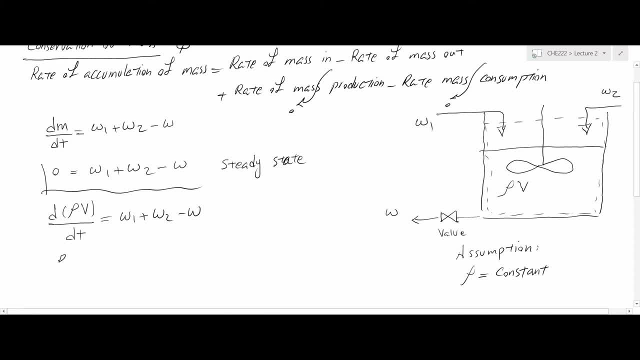 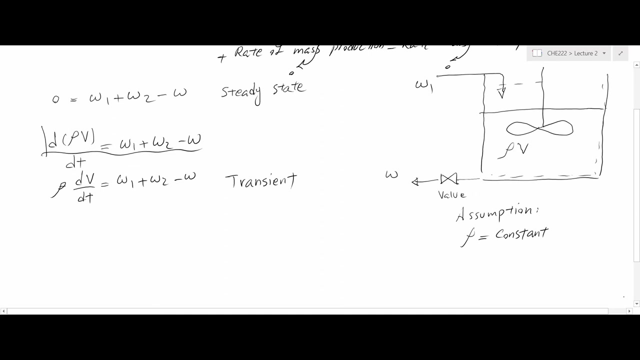 liquids because they are incompressible. so I can take the rho out of the derivative with derivative of volume within the tank and the right hand side stays as is. so this is the conservation of mass in the transient situation of the system. now we can write down the conservation of component. 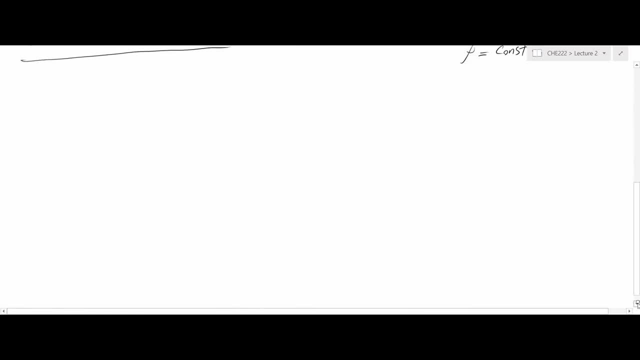 but for that I have to adjust the example slightly. so I will have the same stir tank for blending, but that the inlet. instead of having a pure liquid, I will have a mixture of component a and b. the flow rate will be still w1 and the mass fraction of 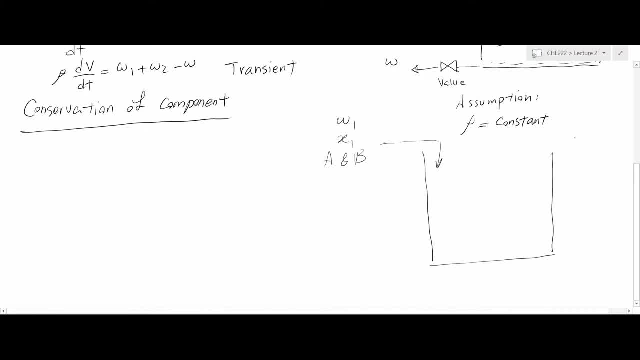 component a is x1. at the stream 2 I will have the flow rate of w2 and the mass fraction of component a is x2. Then the agitator will be here and then at the outlet the flow rate will be W and the mass fraction will be X. 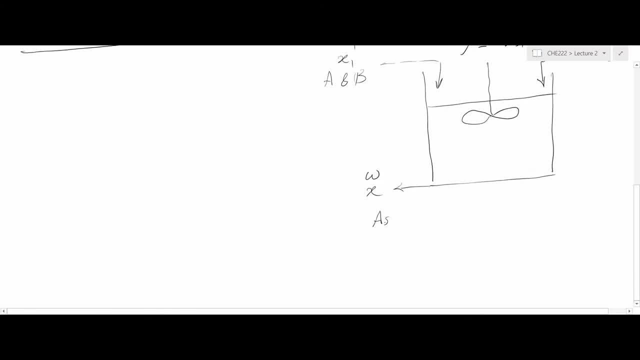 So now I have to make another assumption in here, which is basically ideal blending within the tank, And it means that everywhere within the tank the mass fraction of component A will be uniform because the blending is ideal. So the mass fraction within the tank and the mass fraction at the discharge will be the same, X. 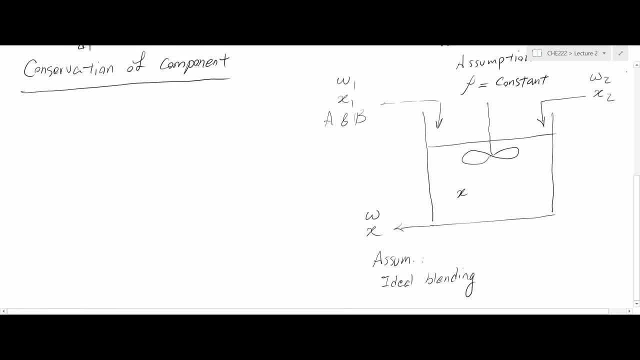 So with that I can start writing the conservation of component And if you remember, we had the accumulation of component or accumulation of any property, in this case component, So I can write that. So I have D over DT of component within the tank, which is total mass within the tank times the mass fraction of component A. 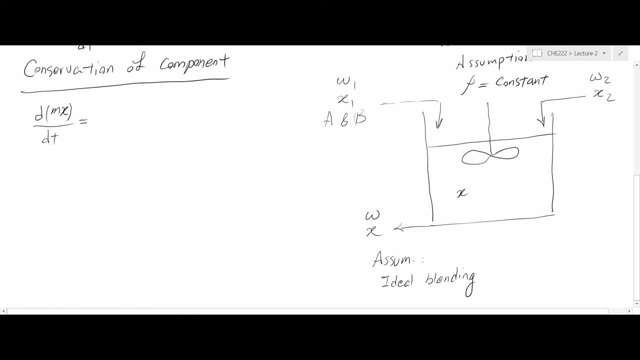 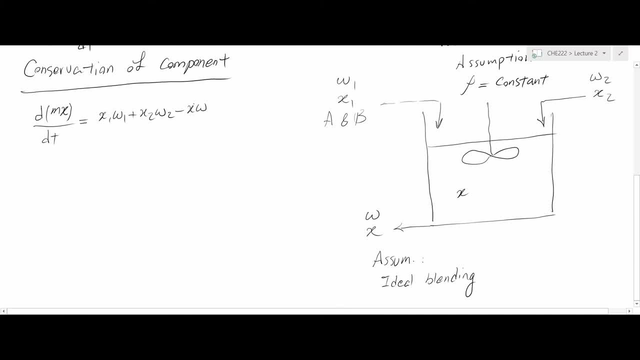 And rate of component out of the tank And rate of component out of the tank. And remember we have production of component and consumption of component. for mass, These two terms, they were zero. But here we may have some chemical reactions that produces a component or consumes a component. 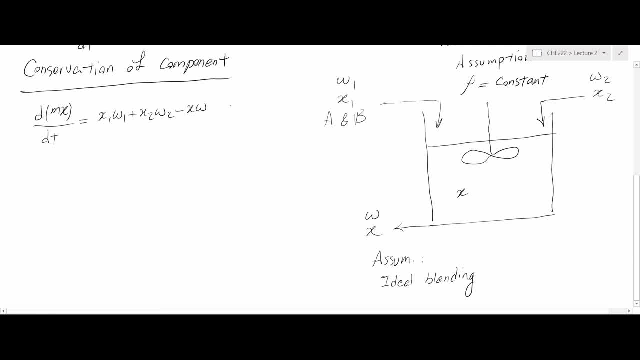 So we will. we may have these terms in future, But as of now this is just pure blending. There is no reaction, So those two terms will be zero. Then I can even make it simpler if I assume again that rho is constant for this: 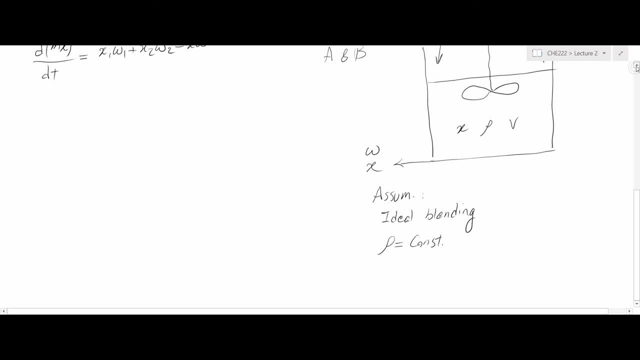 And basically the reason for that would be: if the effect of mass fraction of component on the density is negligible, we can assume that rho is everywhere, is constant. So we can replace mass by rho density times volume. And then in that case, because rho is constant, 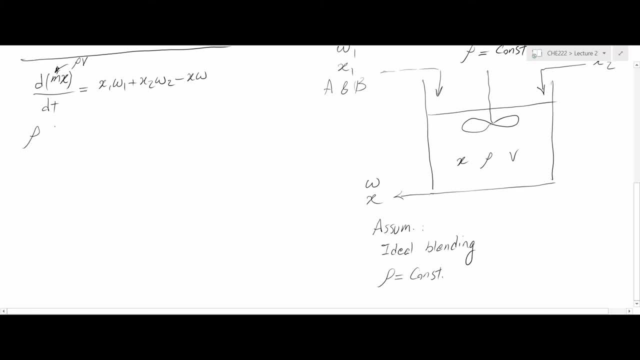 we can factor it out. So we will have dvx dt and the right hand side will be the same: x1w1 plus x2w2 minus x1w2.. And now I can use the chain rule to split this term. 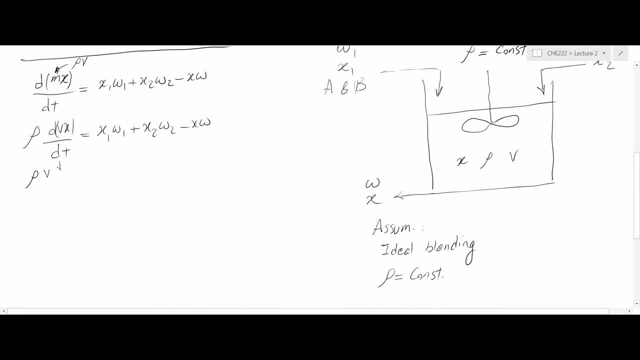 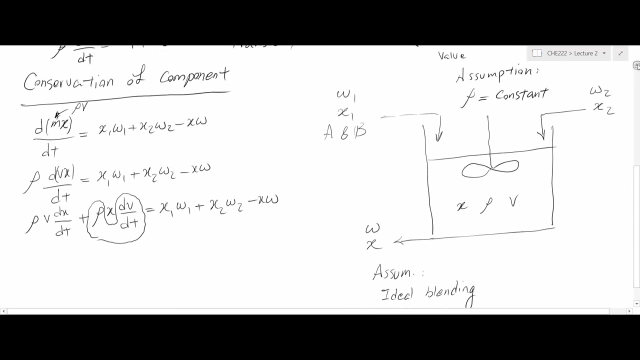 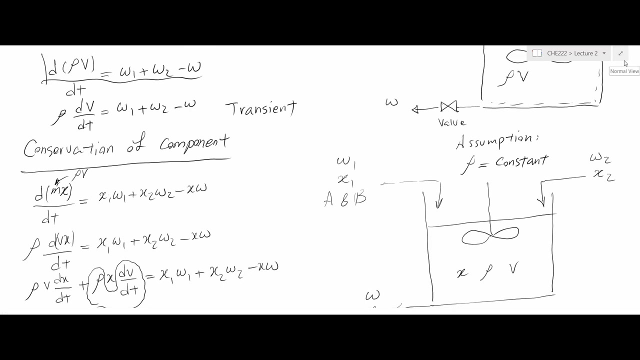 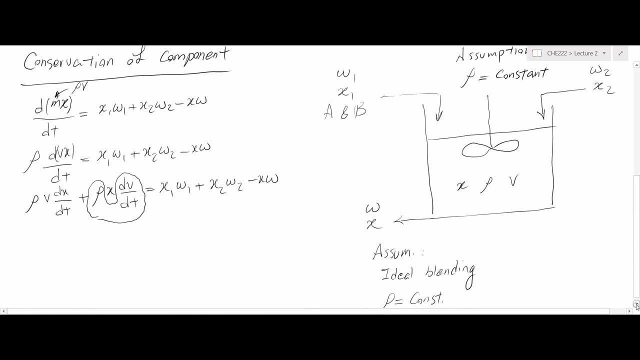 So I can write rho, vdx, dt plus rho, xdvdt equals x1w1 plus x2w2 minus xw. And if you look at this component, this is basically the left hand side of our conservation of basically mass. So we can replace it with the right hand side. 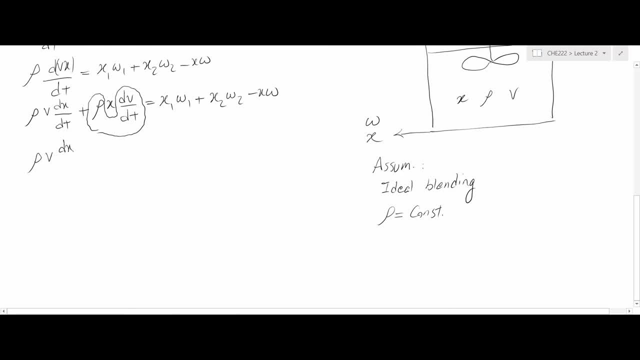 And that's why we will have rho, vdx, dt plus xdvdt. So you're going to have this times: w1 plus w2 minus w is equal to x1w1 plus x2w2 minus xw. And if you rearrange this,